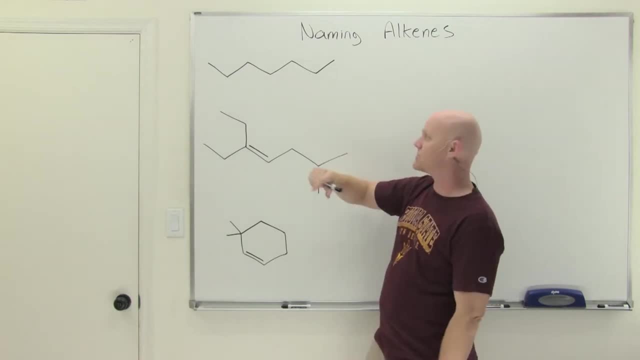 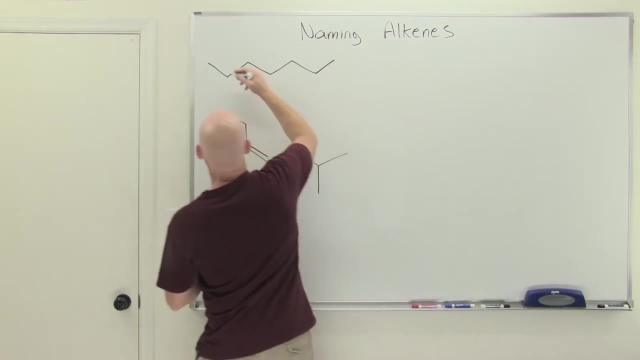 yet. I will add it in a sec, But if you are going to name this as an alkane, just as a review, so it's got 1,, 2, 3, 4, 5,, 6, 7 carbons and that would simply be heptane. So what happens when you? 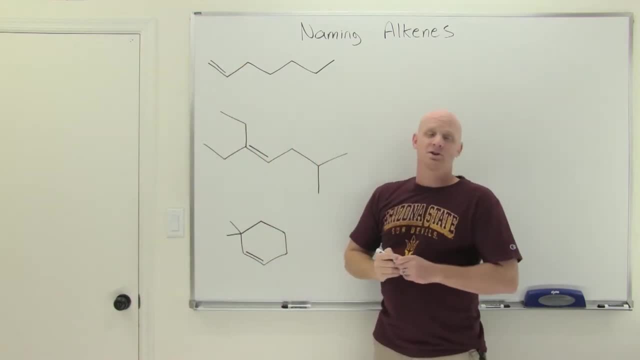 have a double bond, so it's going to be named as part of the parent chain. So, but for alkenes, you're going to have a carbon-carbon double bond, So you're going to have a carbon-carbon double bond. 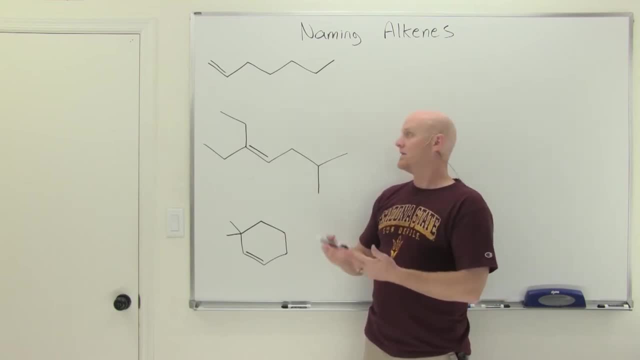 So instead of saying ane at the end of the parent chain, you're going to say ene, And so instead of heptane, this is going to be heptene. So, but it turns out that is not sufficient. So, because the 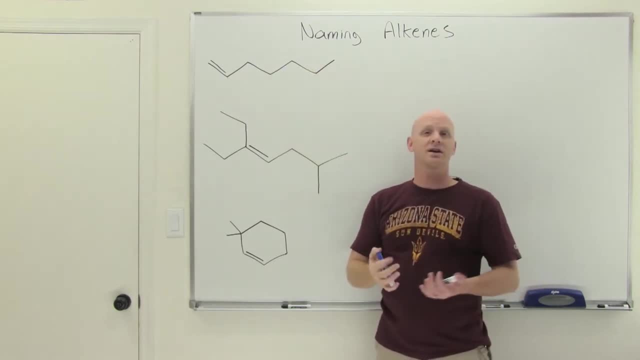 double bond could have been located in one of several different positions, And so you actually got to give a use a chain locator to identify its position as well, And so in this case you find your longest continuous chain that contains the carbon-carbon double bond. Usually it's your. 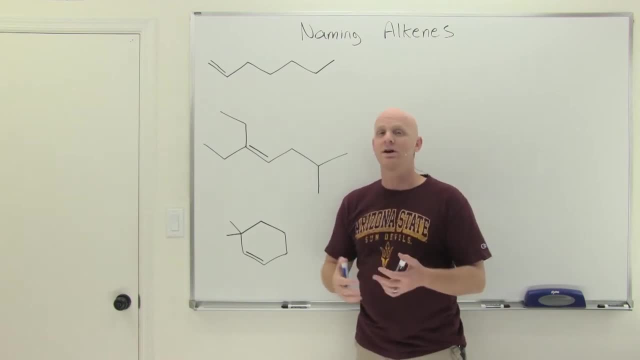 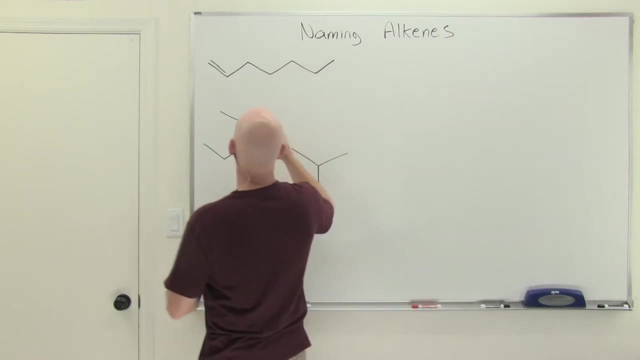 longest continuous carbon chain overall, but that doesn't necessarily have to be the case here. You want, specifically, the longest continuous carbon chain that your alkene is a part of. So all right, then you want to number it in such a way to give it the lowest possible. 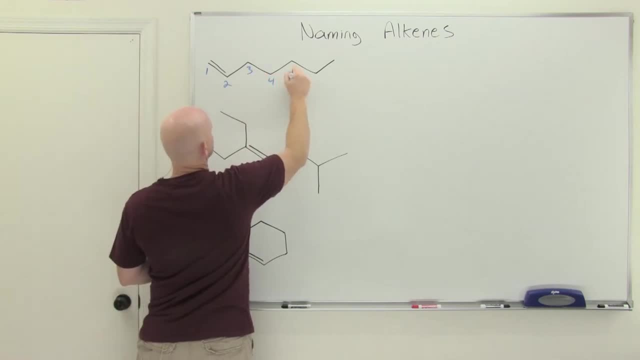 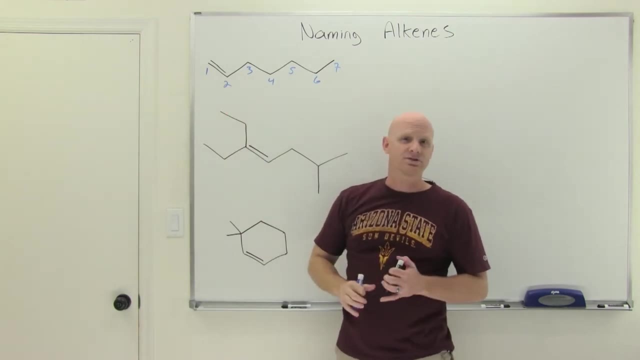 number. So here one, two, three, four, five, six and seven, And in this case the alkene is between carbons one and two and you always give it the lower of the two designations. So it's going to. 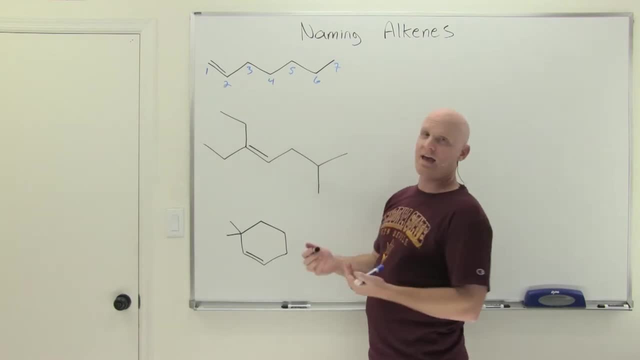 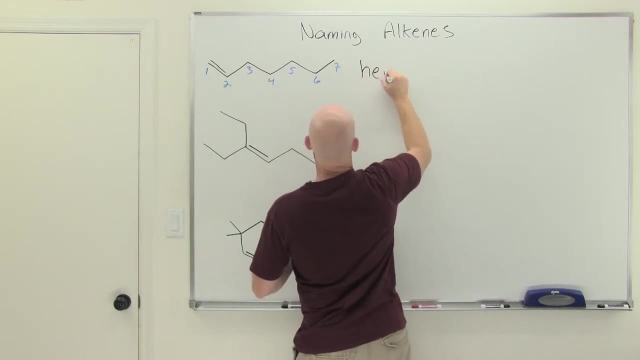 be located at position number one. And so, instead of saying just heptane, like it was an alkane, and instead of just saying heptene, which doesn't give us chain locator, we're actually going to say hept, dash one. 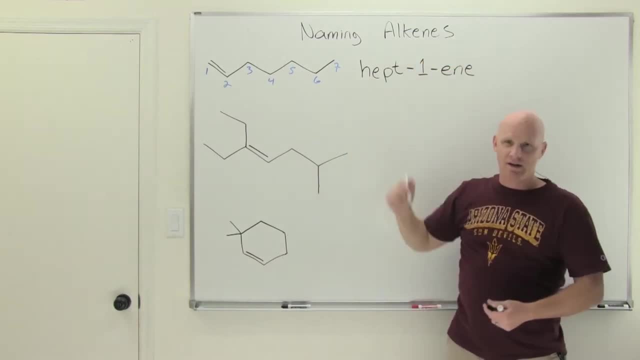 dash in. This is the most accepted way, So you'll find out. usually acceptable also, though, in this case, is to say one dash heptane as well. So you'll find out, when you've got multiple functional groups that are part of the parent chain's name that you're going to get stuck. 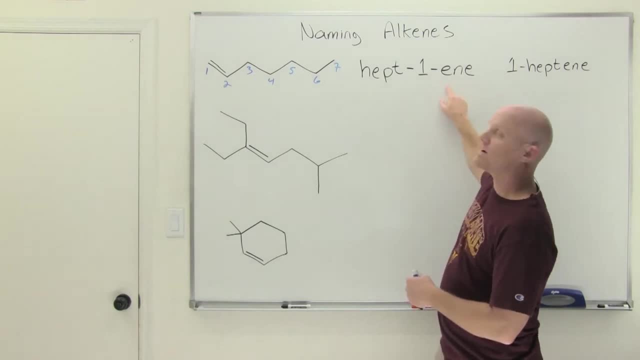 putting the number in the middle of the word right before the little suffix here. that identifies it as an alkene. So, but if the alkene is the only major functional group in your parent chain, then you can actually put the one out front, as I've done there as well. 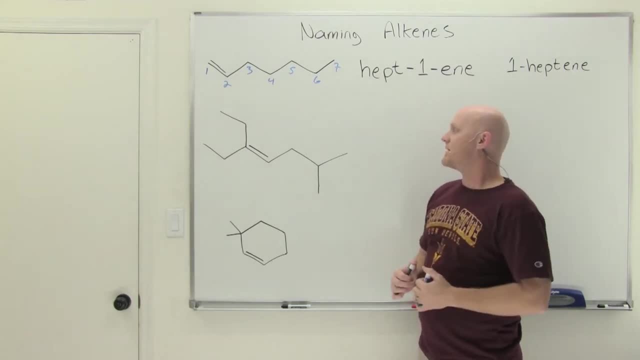 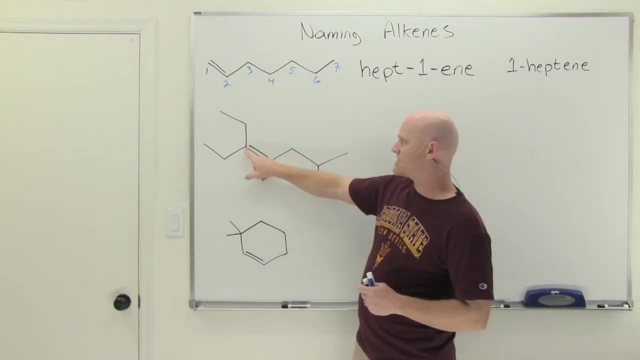 All right, So that's the first one. Start off easy, Let's make this harder. So next example: find your longest continuous carbon chain that the alkene is a part of. And so, in this case, starting from this branch, point here whether I go to these two carbons or to these two. 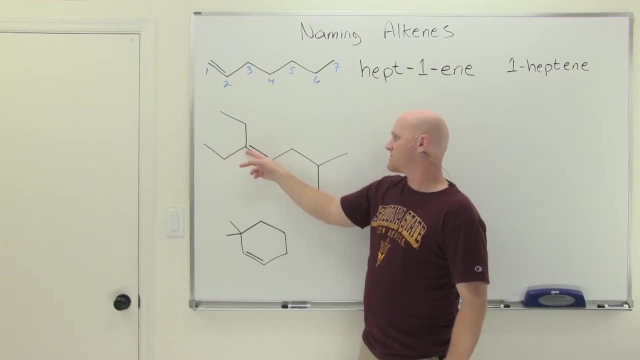 it is the same length either way, It doesn't make a difference. So, in this case, one, two, three, four, five, six and again. whether I go up or down doesn't matter. So, and that'll be the, 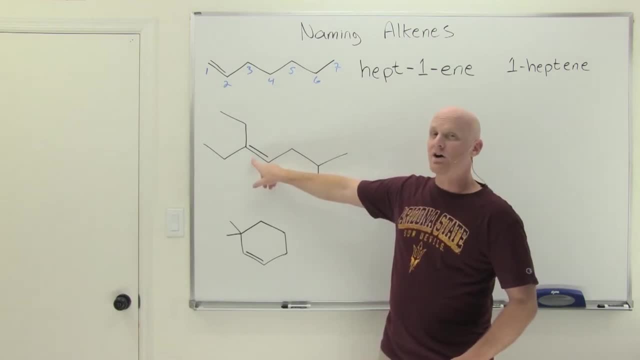 seventh, And in this case when a number, it's such a way to get the alkene the lowest possible number. So in this case, one, two, three, or one two three, four, five, six, five, six, five, six. 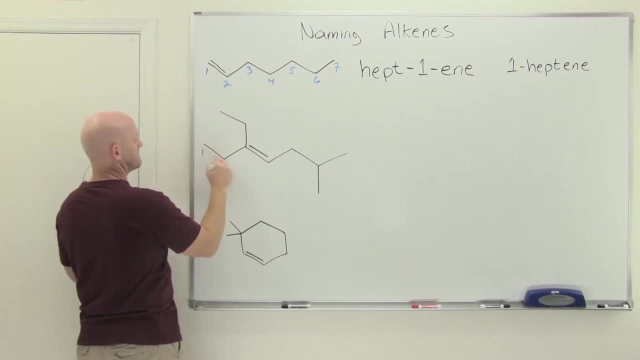 four. So we'll number left to right, give it that lower number three, Cool. And then we start this out just the same way. we name alkanes and you name all the substituents first, And so, in this case, what's not part of that parent chain? Well, we have got. 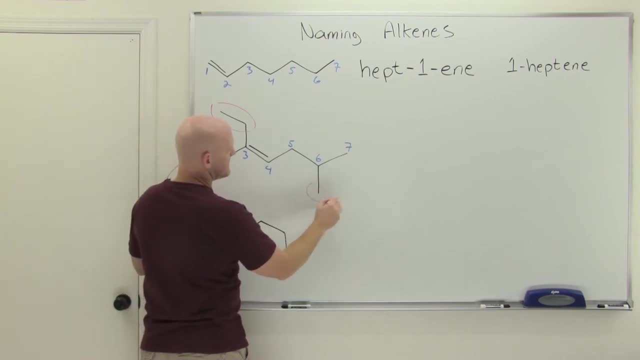 an ethyl group right here on, attached to carbon three, and then we've got a methyl group down here attached to carbon six, and you name all your substituents in alphabetical order, So we'll name the ethyl first, And so in this case we will say: 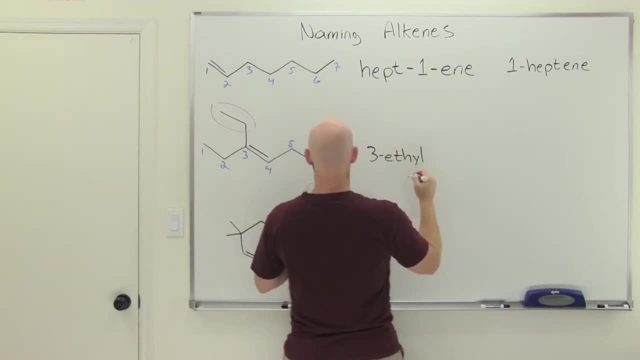 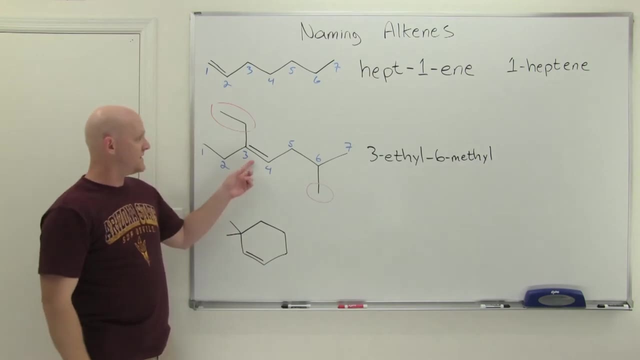 three ethyl, then six methyl And in this case, to name that alkene, again, you're going to give it the lower of the two numbers. It's between carbons three and four, So we're going to name it as being at position three. 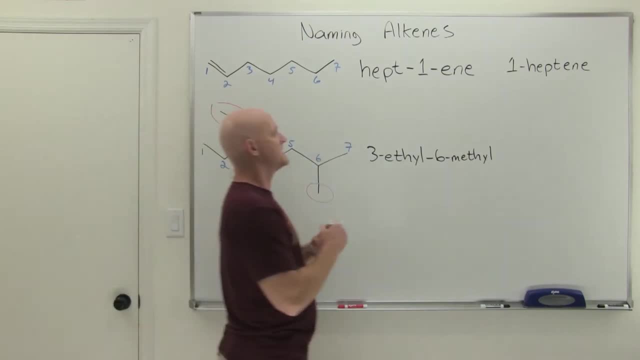 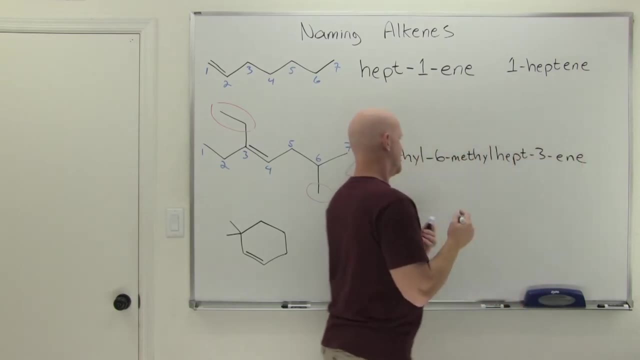 Longest chain is seven carbons again, So it's going to be heptene. But instead of saying heptene, we got to give that chain locator again, So we'll say hept, dash, three, dash, ene. Now in this case. 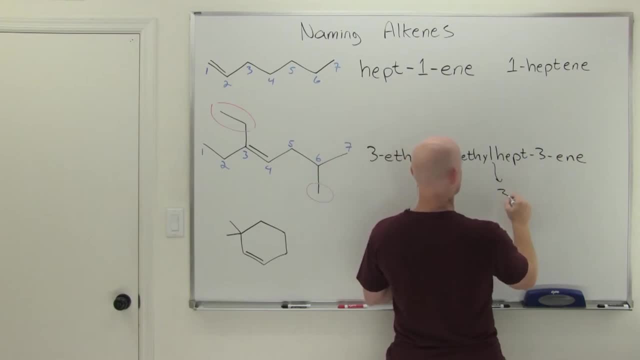 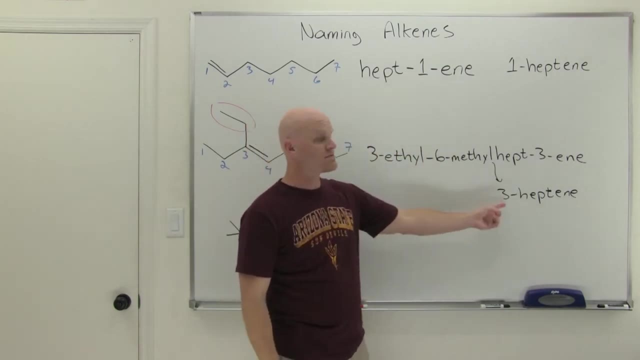 we also could have set it one other way here and we could have said three heptene as well at the end. So it would have been three ethyl, six methyl, three heptene, And most professors have no problem accepting either one of those as acceptable IUPAC names. 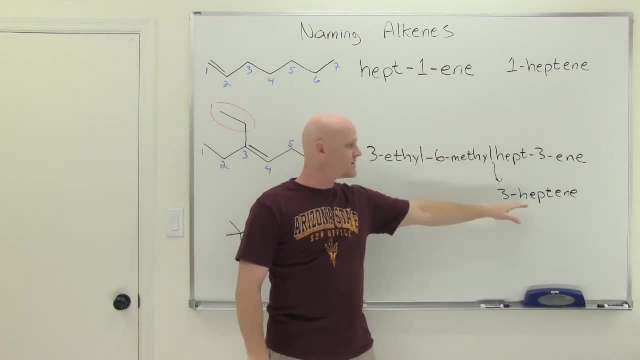 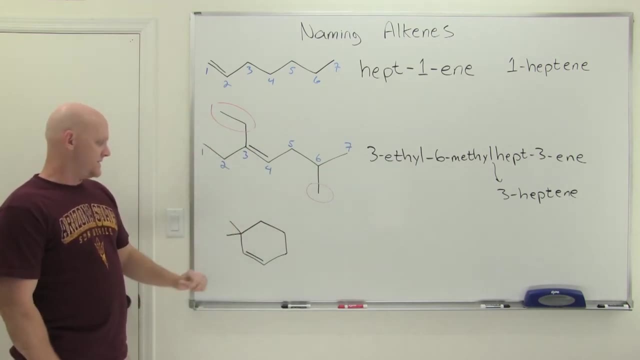 So, but you'll find that the top one, though, is kind of the more proper- This is kind of the old school, but the more proper. but again, both should be acceptable, All right. So what if we got a cycloalkene in this case? So if you've got a cycloalkene- assuming the alkene is the most- 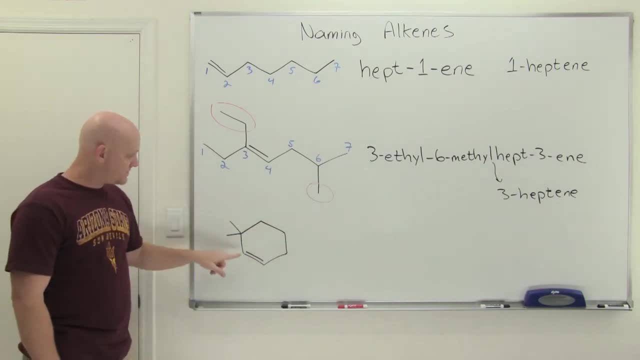 important function. you're going to get a cycloalkene. So if you've got a cycloalkene in your ring, then those two carbons have to be carbons, not just one but one and two You have. 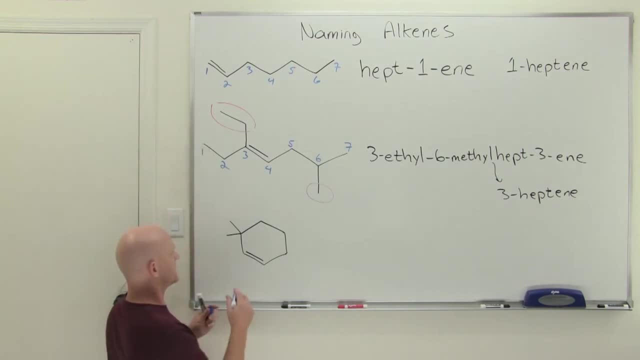 to number through that alkene, And so the question then becomes: do I want to say like one and two, or do I want to go one and two? So one of the mistakes students make is they often don't realize that they actually have to make these the first two carbons Like they want to start. 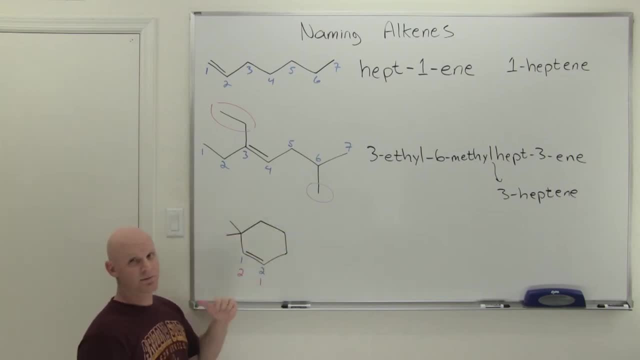 with him as number one and then number around this way to get the substituents the lowest number. but it's both carbons of the alkenes that have to get the lowest and that's why you got to number through. So, but in this case, whether it's one and two or one, 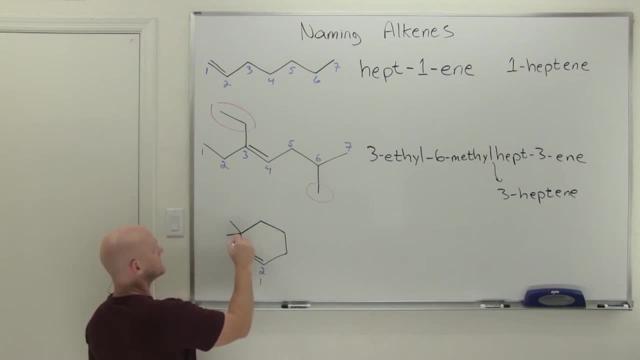 and two makes no difference as far as the alkene goes, but it will make a big difference for our substituents, And so in this case we're going to number this around clockwise, as we did in red here. So one, two, three, four, five and six, And we will name this, the substituents, first again. 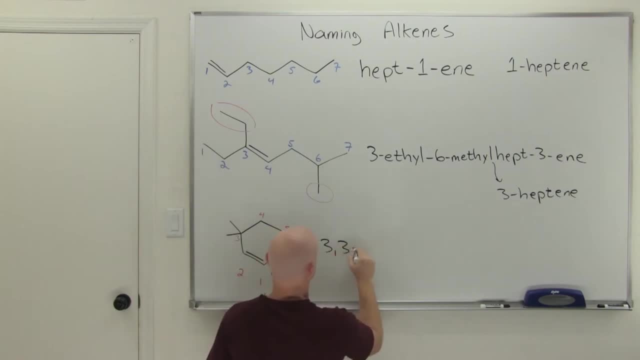 So three, three dimethyl, All right, And then this is cyclohex- not ane, but cyclohexene, So, and what you'll find here, though, is that, if you're naming it cyclohexene as your parent chain, 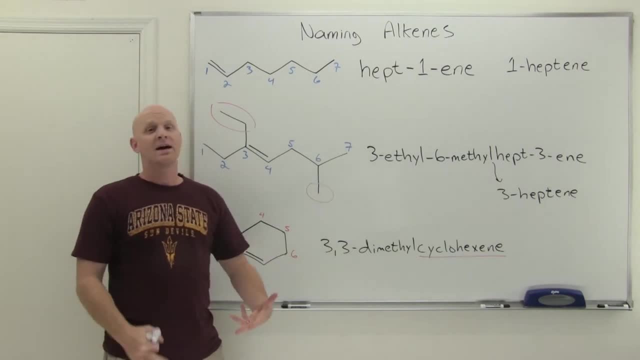 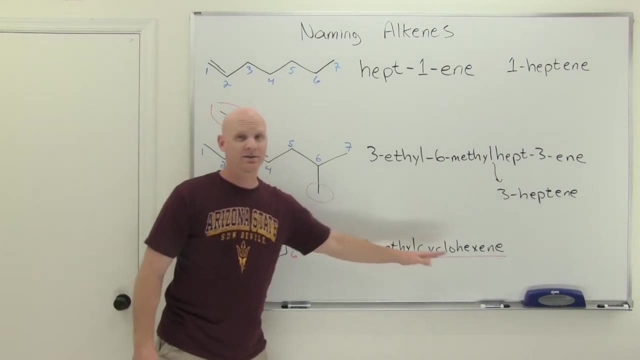 well then, the alkene is the only functional group in that parent chain And therefore, by definition, in a ring, it would have had to bend between carbons one and two and been at position one, And when that's the case when it's cyclic notice, this wasn't the case when it was on an 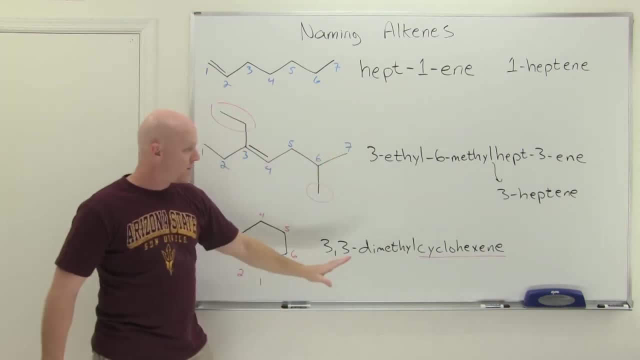 open chain. when it was in a ring it would have had to bend between carbons one and two At position one. we had to include it as part of the name. but when it's in a ring here, you don't include it as part of the ring. It's totally implied. So no chain locator, It's not. 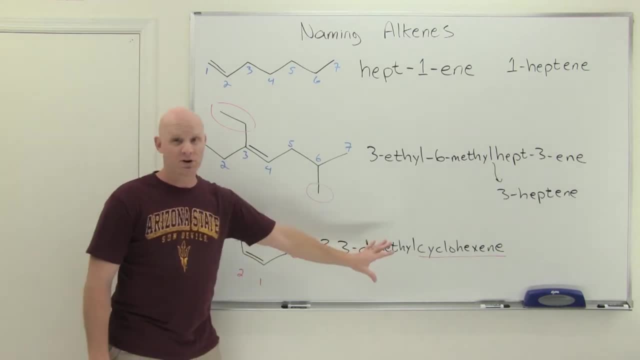 that those chain locators needed, it's that you don't put it in. If you put it in there, you might lose half a point on something like this. All right, So now let's talk about stereoisomers. So reminder, the carbon-carbon double bond in alkene is not free to rotate. You've got that. 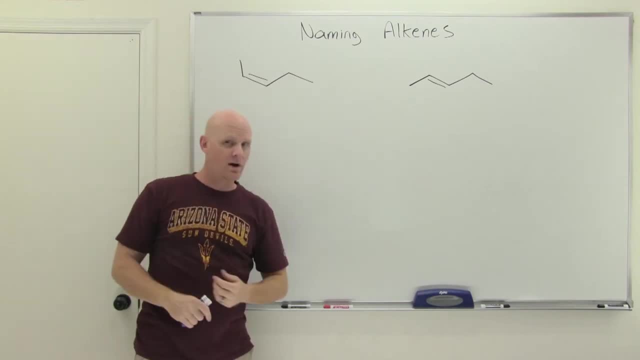 sideways overlap of p orbitals And if you rotate the bond you'd break the double bond. So no rotation here And that leads to different stereoisomers being possible. So in this case you guys learned back in the chapter on stereochemistry that cis and trans isomers were possible with alkenes. 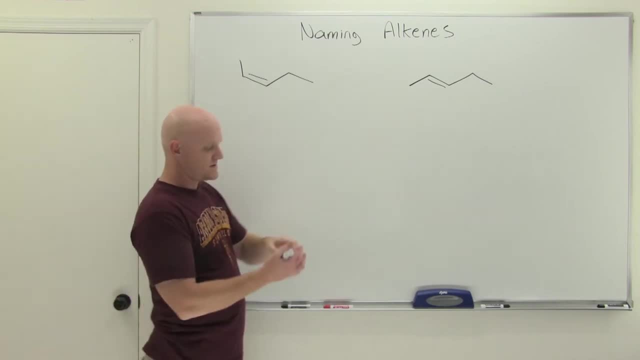 and that they are diastereomers, as is the case here. So, and back in the day, we were referred to this one as cis and this one is trans, but that actually is not going to be good enough, That's not going to be quite enough, because the cis and trans- here you got to talk. 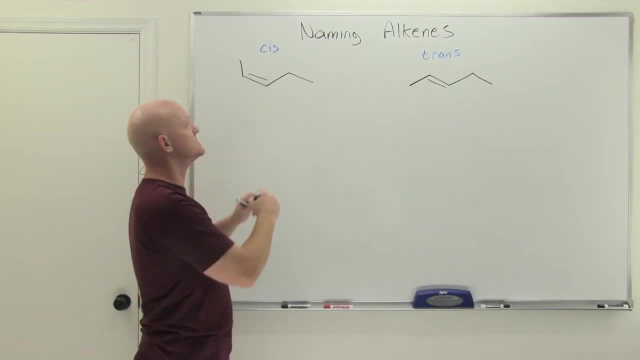 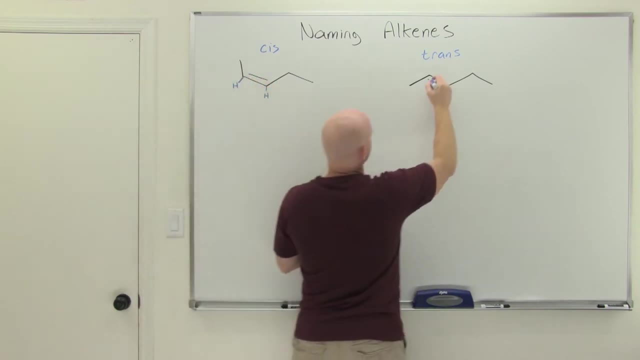 about what actually is cis and what actually is trans. And in this case we actually could use it If both of the carbons of the alkene have a hydrogen- and I'll draw those hydrogens in that weren't drawn and they each got one. And if they've got one each, you can actually use the cis and 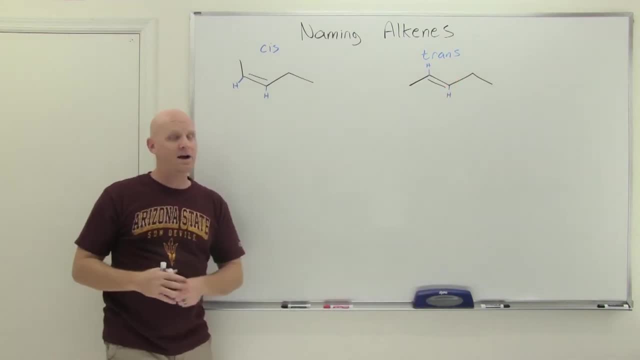 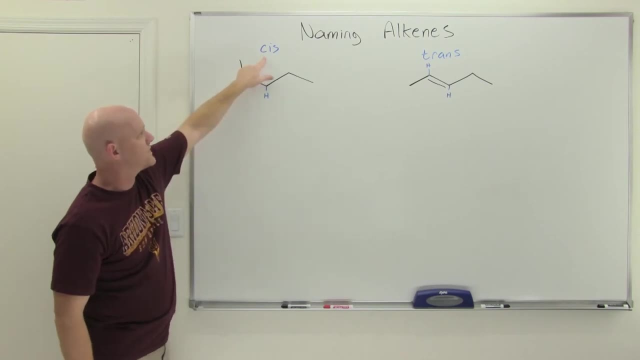 trans system of nomenclature. It's not proper, It's not IUPAC, but you can use it. So in this case, if you look at, the two H's are only pointing 60 degrees apart, and that's when it's cis. 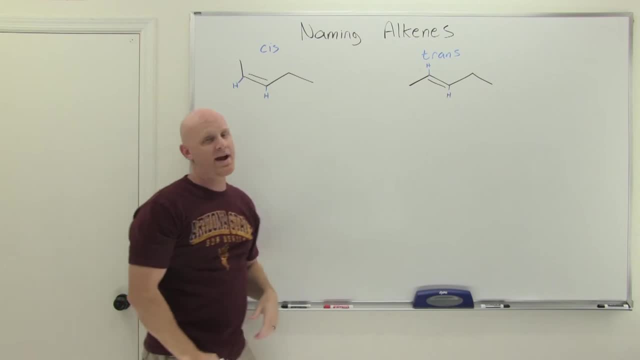 but when they point 180 degrees apart, that's trans. So but what if both sides don't actually have an H? So that's one problem. So, and then to recognizing when you've got to use cis or trans, or what we're going to call E and Z. So, but it turns out that, you know, not all alkenes actually. 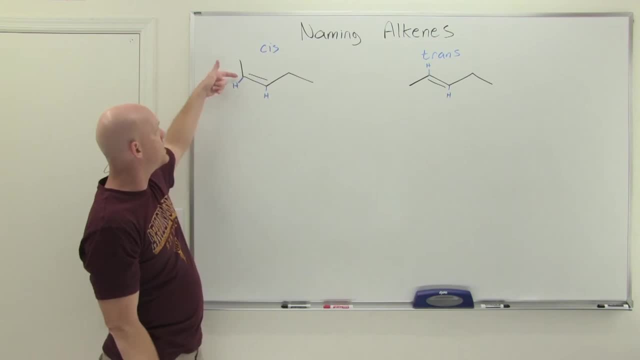 exhibit cis trans isomerism. So as long as both sp2 carbons of the alkene are bonded to two different groups, it'll be capable of exhibiting cis trans isomerism. or if it's not, part of a smaller ring. So if it's in a smaller ring it's just going to be in the confirmation that's in. 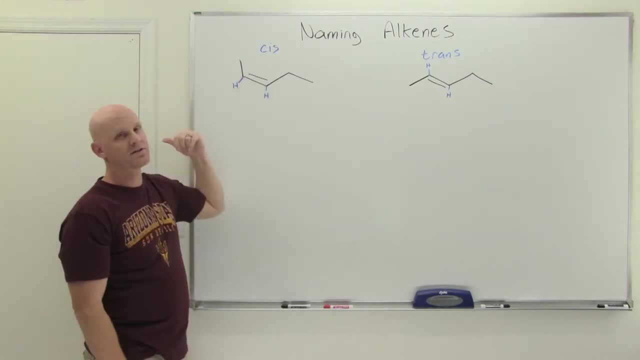 but it's in a larger ring. Or again, if both sp2 carbons are bonded to two different groups, it will exhibit cis trans Isomerism. So in this case, sp2 carbon on the left is bonded to a carbon of a methyl and a. 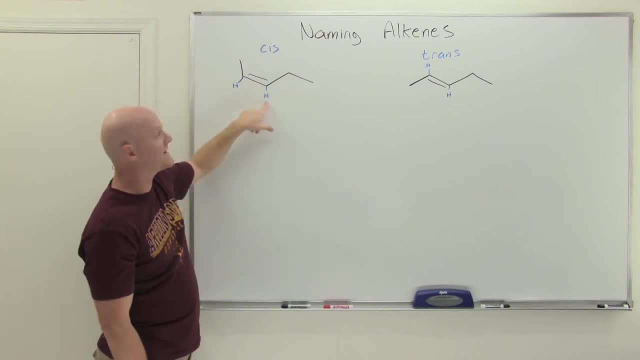 hydrin. So sp2 carbon on the right is bonded to the carbon of an ethyl and a hydrin. Both sp2 carbons are bonded to two different things And yes, indeed, we're going to have cis trans isomerism And all you got to do to get the other isomers, take either side and have the two groups. 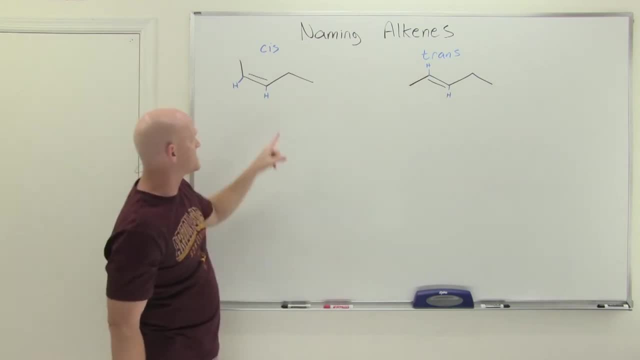 trade places, which is what we've done to get the trans isomers over here. So I left these two alone: the ethyl and the hydrin on the right-hand side just had these two trade places. So, but instead of cis and trans, we're actually going to use what's called E. 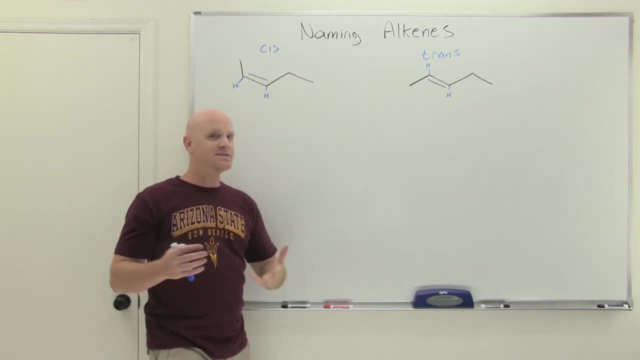 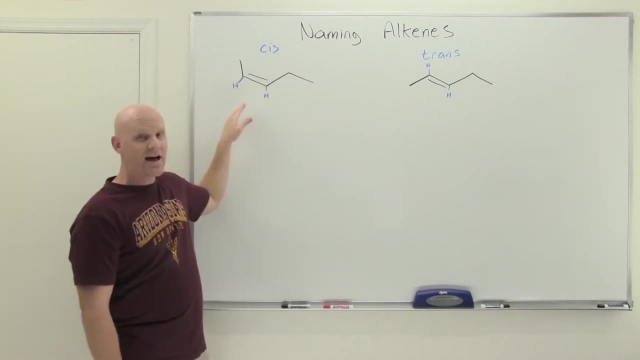 and Z And the E. there are a couple of German words, entgegen and zusimon, and it doesn't matter, So, but E is going to be analogous to trans and Z is going to be analogous to cis, And I like to say that your two, like priority groups, are on the same side. So it's the stupid. 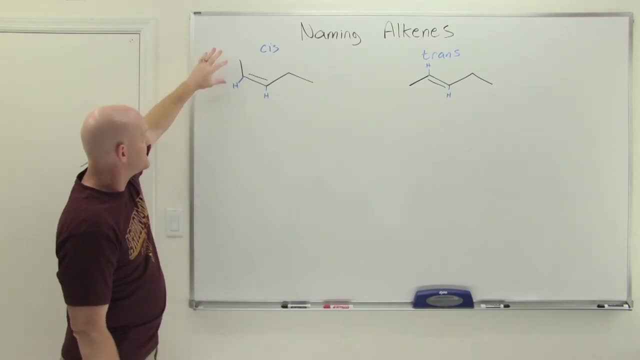 mnemonic. we kind of emphasize there the alliteration. So in this case, what you're going to do is actually assign priorities, So to the two groups, a higher and a lower- and, truth be told, we're just gonna really worry about the higher. So, and it's the same way you. 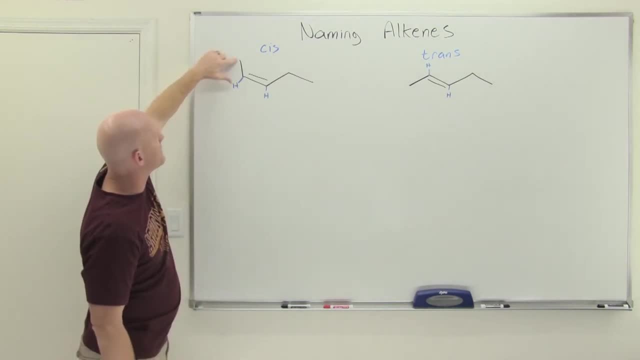 assign R and S. So in this case to this sp2 carbon. it's bonded to a carbon and a hydrin. Carbon's got the higher atomic number And so it's going to have the higher priority on the other side. So again, hydrin versus carbon, carbon has a higher atomic number, So that group is going to. 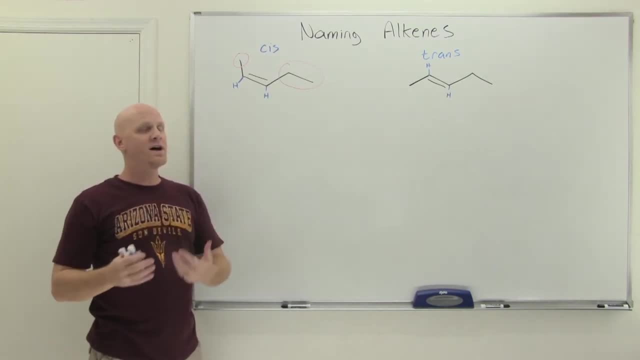 get the higher priority, just like we assigned priorities with R and S. but instead of deciding like four priorities, each side just has a higher and a lower and just circle those hires, You relate those two And when those two higher priorities are on the same side, when they're. 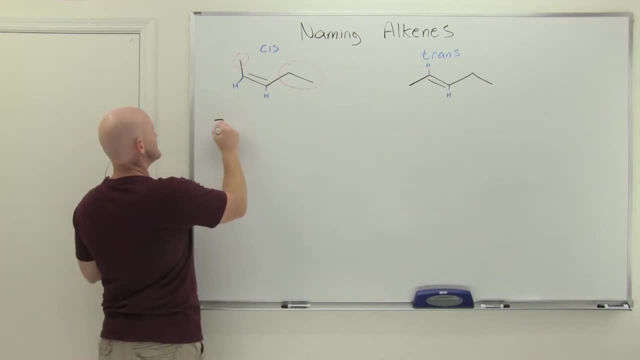 cis to each other. we will refer to that as the Z isomer And we'll put that out in front in parentheses, just like we'd put R or S out in front when we're naming stereoisomers that have R and S- chiral centers. So, and in this case then we'll name the rest of this and this alkene. 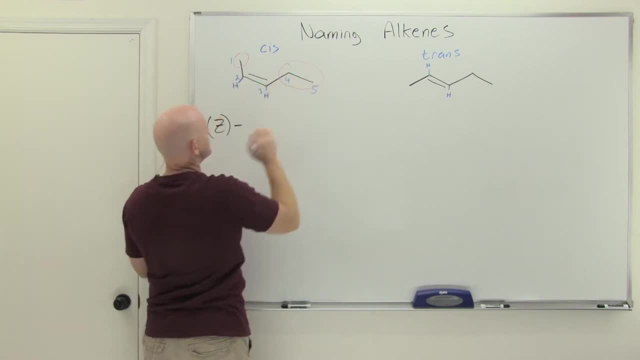 one, two, three, four, five, name to get the alkene the lowest possible numbers, And in this case this is pent-2-ene or 2-pentene, but I'll call it pent-2-ene. So Z, pent, two. 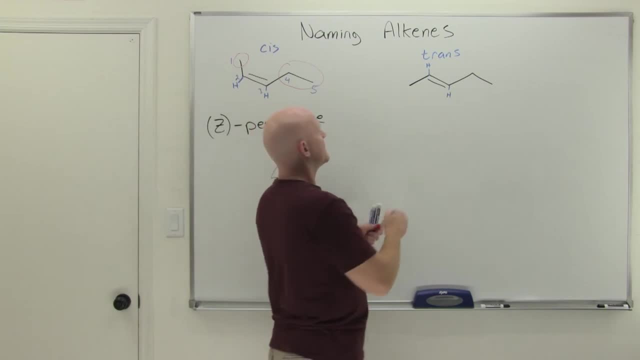 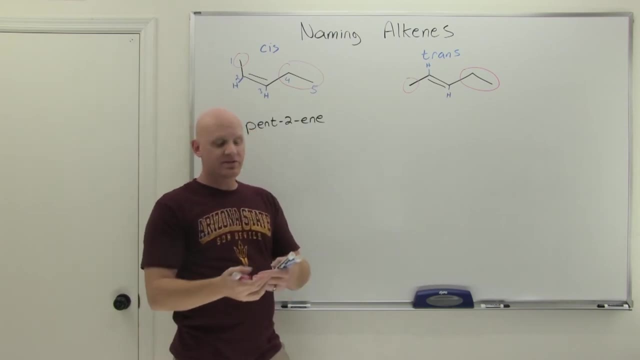 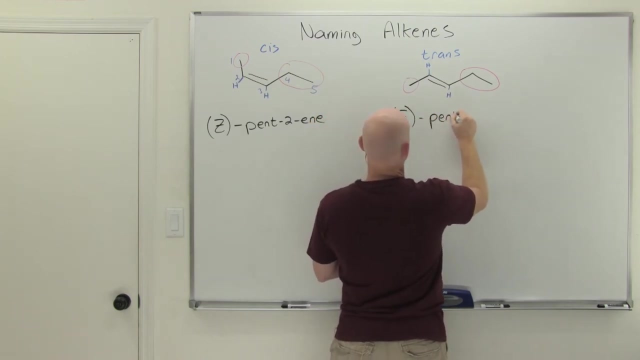 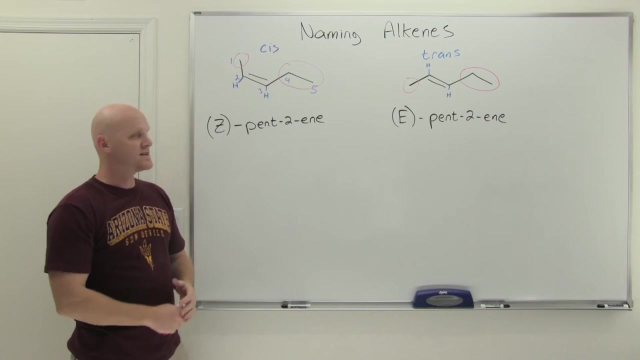 in Cool. Now, on the other side here, if we circled again those high priority groups, they would now be trans to each other. So they're not cis, they're trans. and that corresponds to E- Cool. So and that's how the nomenclature kind of works with E and Z. So one. 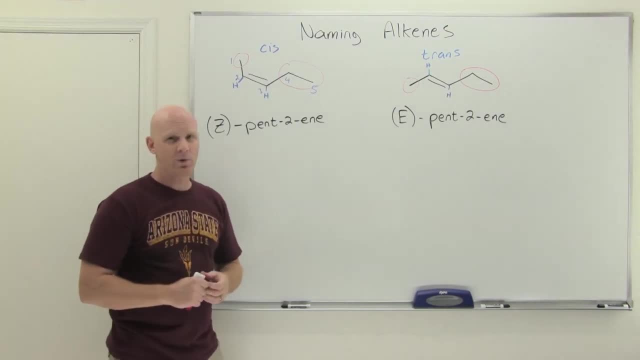 you got to kind of, you know, drug up those con-engled pre-log rules for assigning priorities. Then relate your two higher priority groups. If they're only 60 degrees apart, that's going to be cis, which now corresponds to Z as the proper IUPAC name, And if they're 180 degrees apart, 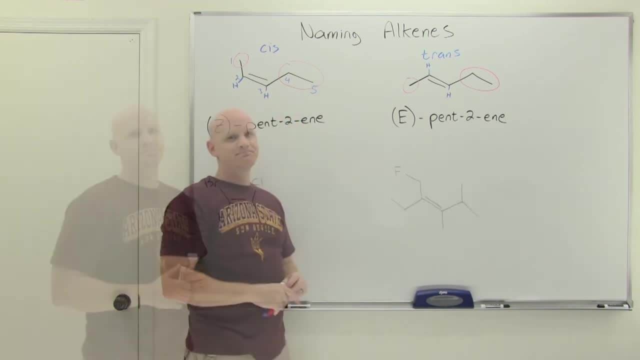 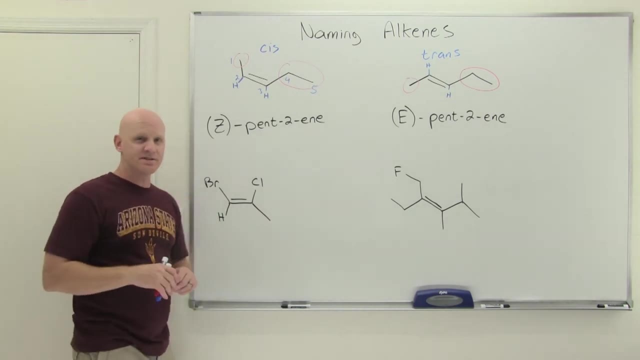 which was trans. that's going to correspond to E as part of the IUPAC name. All right, for these next two. we're not actually going to name these two. I just want you to assign E and Z. So you might take a moment and pause this and assign E and Z and we'll measure it. 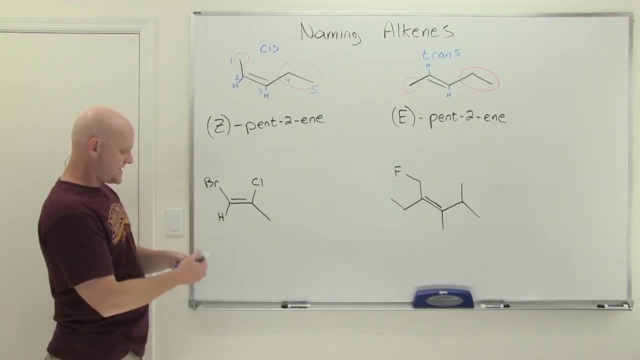 up together. Now, the first one here is easier than the second. So if we take a look again, those sp2 carbons- the sp2 carbon on the left is bonded to two groups of bromine and a hydrogen. The bromine's got the higher atomic number. Life is good. And on the right-hand side, 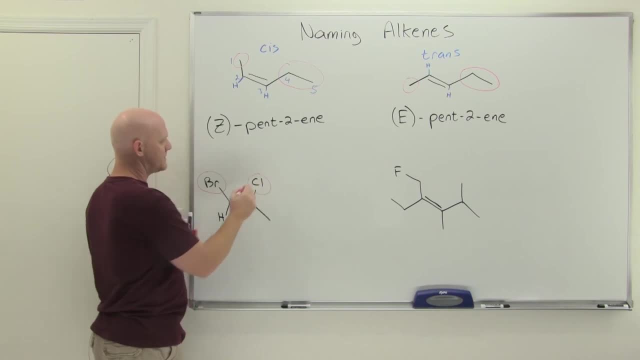 that sp2 carbon's bonded to a chlorine and a carbon, Chlorine's got the higher atomic number. And here we can see that the two higher priority groups are only 60 degrees apart. They are cis to each other, ie they are on the same side. They're Z. This is the Z isomer here, in this case. 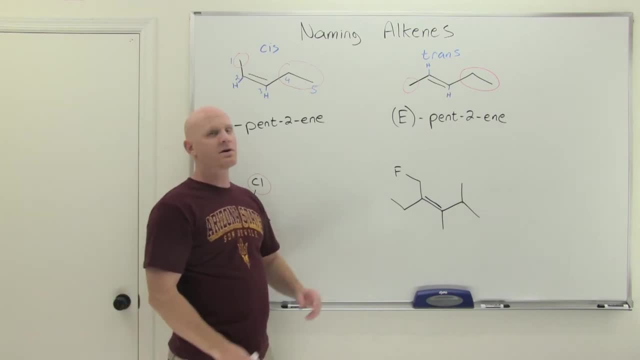 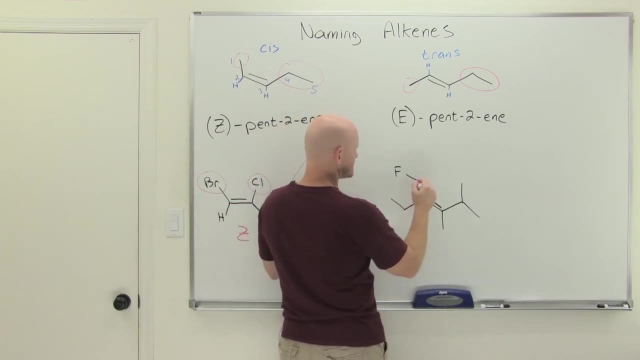 But the next example is a little trickier. We'll definitely need a full application of our con-engled pre-log rules here. And for the sp2 carbon on the left. it's bonded to two identical groups, It is bonded to a carbon and a carbon, And so then we've got. 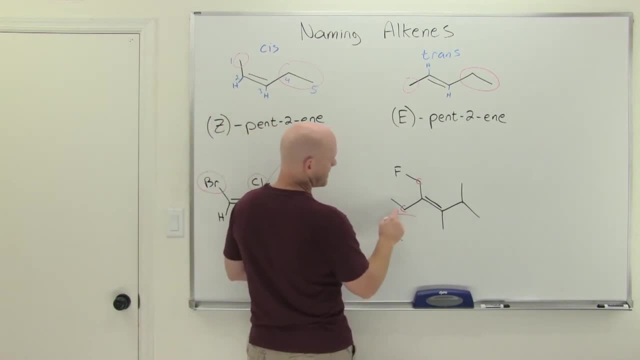 to say: well then, what are those carbons bonded to? Well, this carbon down here is bonded to one other carbon and then not drawn in is two hydrogens. So, in this carbon up here is bonded to a fluorine and then two hydrogens that are not drawn in. And so the first place where they're 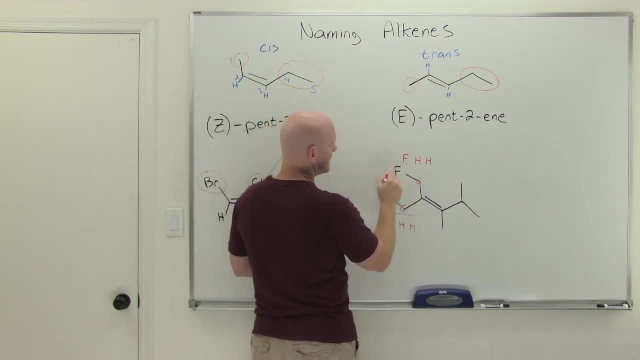 different is comparing carbon to fluorine. Fluorine's got the higher atomic number, And so this is the higher priority on the left-hand side. And then you're right-hand: sp2 carbon is also bonded to two carbons, So there's a tie, So we go further. 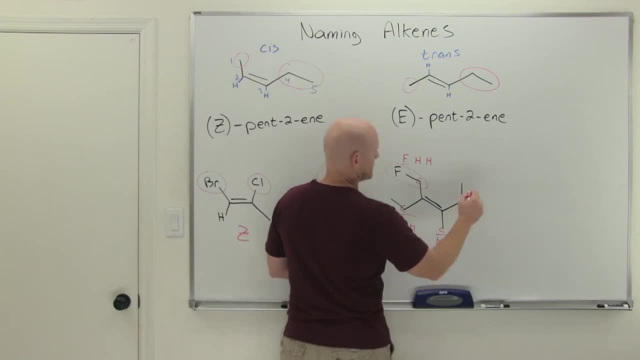 and this carbon down here is bonded to three Hs that are not drawn in, Whereas this one over here is bonded to two carbons and a hydrogen. We can see the first point, where it's different: Carbon's going to beat hydrogen, And so this will be the higher priority group, And now we can see the two. 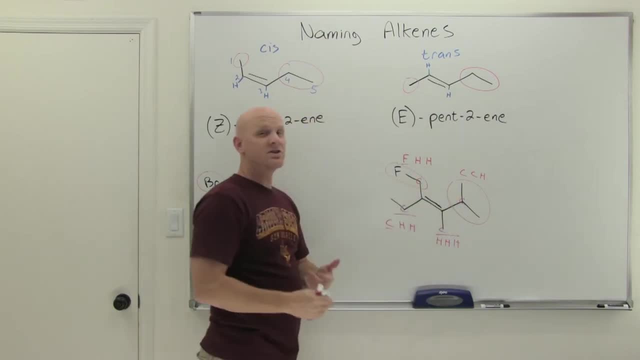 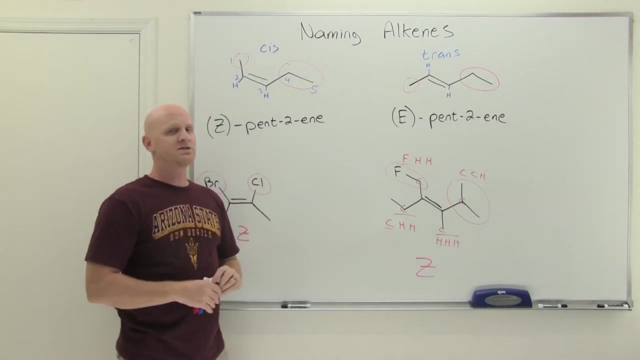 higher priority groups, again only 0.60 degrees apart. They're cis to each other And once again this would be a Z isomer as well. Cool, Takes a little practice, works several examples, but should be fairly reminiscent of what you did with R and S. 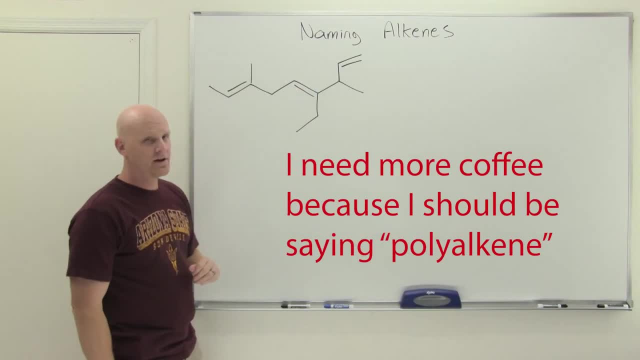 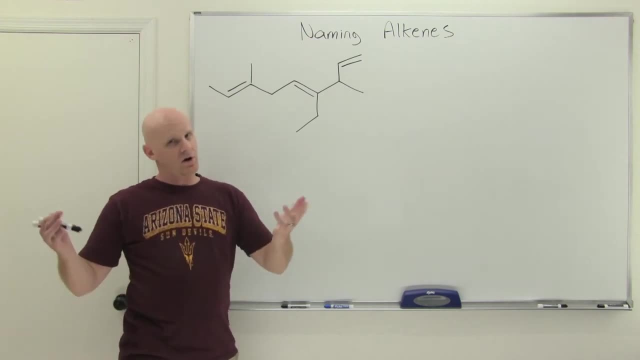 All right For our last example. here we're going to name a polyalkane, And when you've got a polyalkane, you want to find your longest continuous carbon chain that contains all of the alkenes if possible. It's not always possible, but as many as possible is the case here, And so in 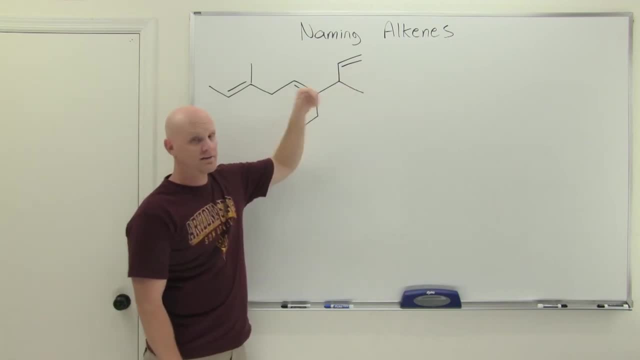 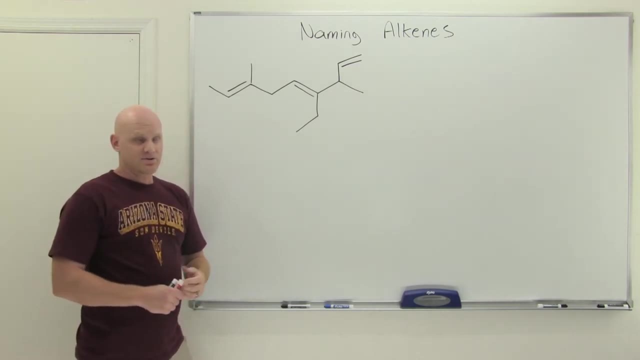 this case we will get a longest carbon chain that does indeed contain all of the alkenes, And so in this case it'll be three alkenes And we'll call that a triene, And that's going to be part of the parent name, So it turns out with: 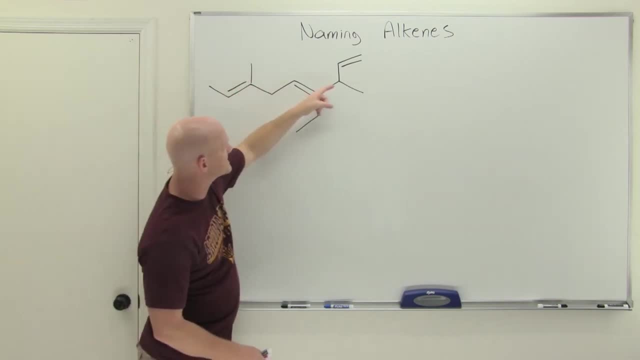 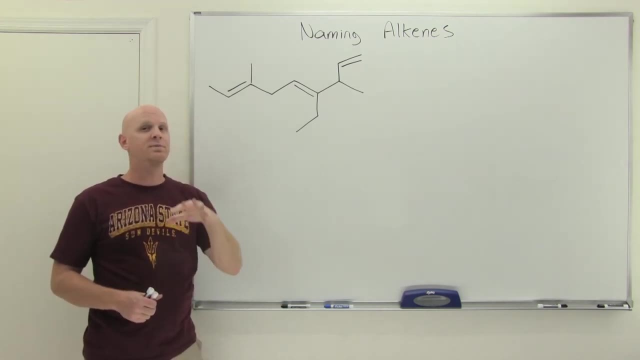 just one alkene you might like, in this case one, two, three, four, five, six, seven, eight, nine. So nonane becomes nonene for a single alkene. But if you had two alkenes it would be nonadiene. 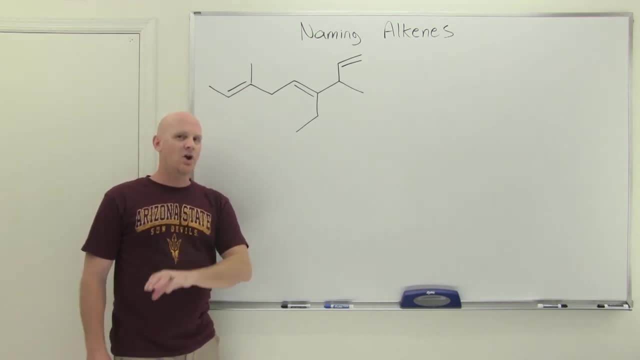 And since diene begins with a consonant, we pull that A back in on nonadiene, so we don't have, like non-diene, a consonant, consonant sound. So it'd be nonadiene, And with three of them here. 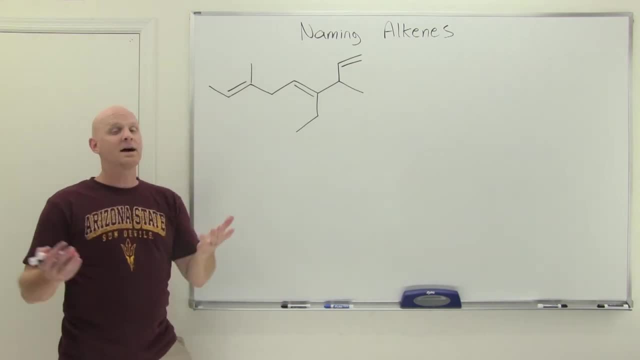 it's going to be nonatriene for the triene, So nonadiene, nonadiene, triene, triene, triene, triene, nonatriene for the parent name, And again we will have to include those chain locators as well. 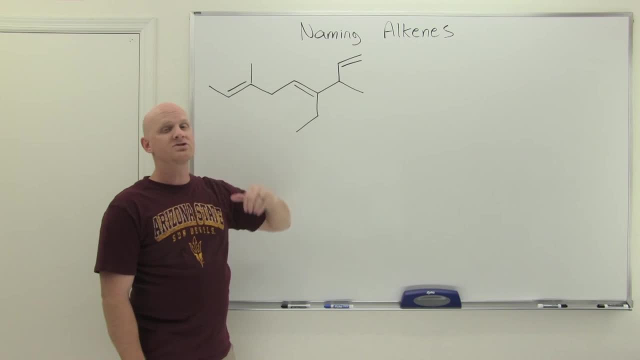 Now, in this case, once we've identified our longest chain, which we just identified as nine carbons, you want to number it in such a way that the first alkene you encounter gets the lowest possible number. So if I go left to right, I will hit an alkene at carbon two, But if I go right to 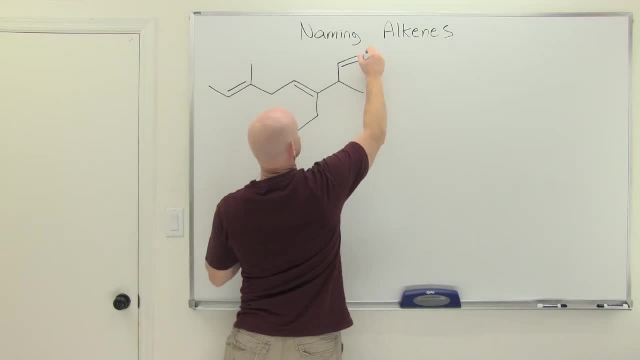 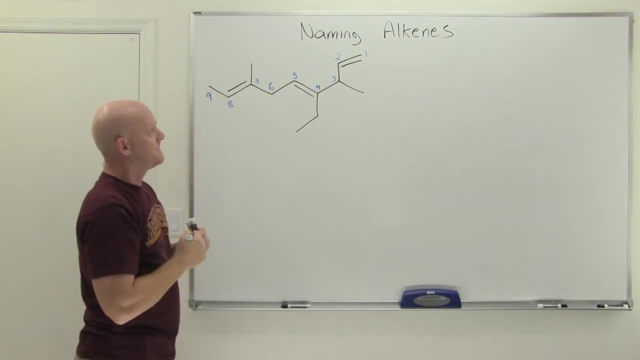 left, I'll hit an alkene at carbon one, And so we'll number this right to left here. So one, two, three, four, five, six, seven, eight and nine. All right, So if we look here, just like normal, we're going to name the substituents first, And we've got. 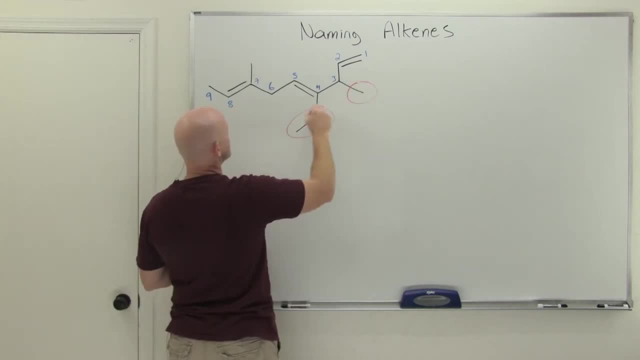 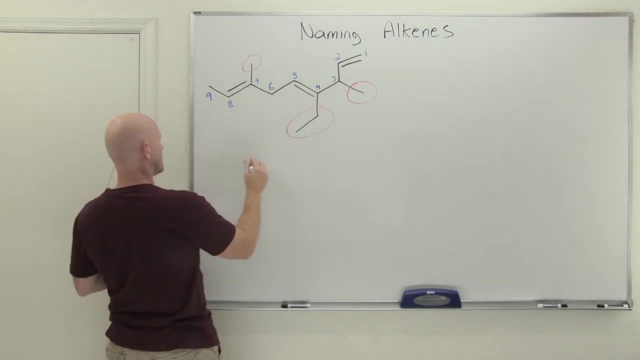 substituents. at carbon three, here there's a methyl. At carbon four, here there's an ethyl. And at carbon seven, here there's another methyl. We'll name ethyl before methyl in the alphabet, And so we're going to say four ethyl, and then three, seven, dimethyl. 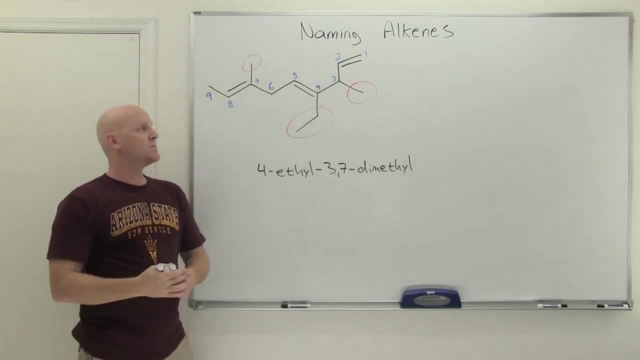 All right, Now the fun. We've got non-triene, But in this case we got to give three different chain locators at position one, position four and position seven, And you're best to put those in the actual word before you. 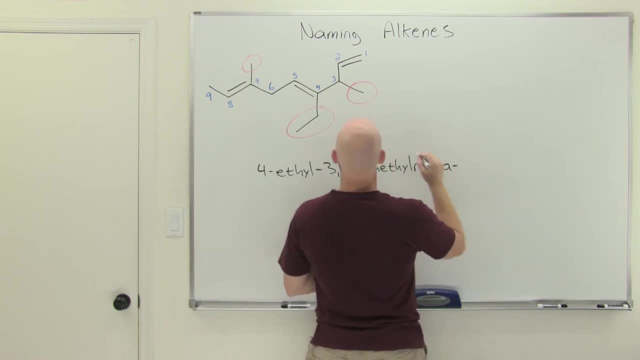 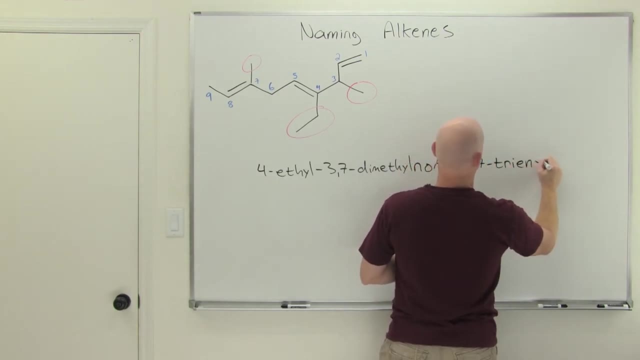 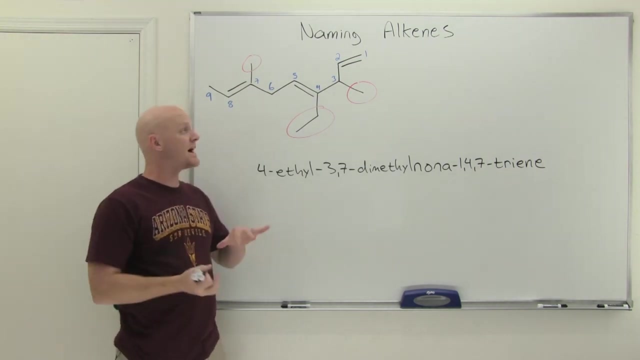 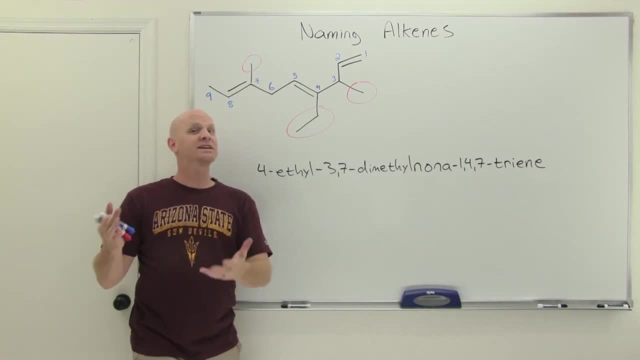 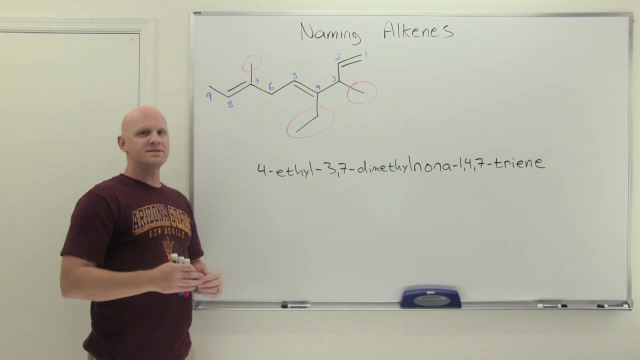 You should check for stereoisomers. Are cis and trans or E and Z possible? And in this case it's not always possible And like we mentioned this before and we didn't kind of point it out explicitly, but the first few examples we gave, if you go back and look at them, so they're either 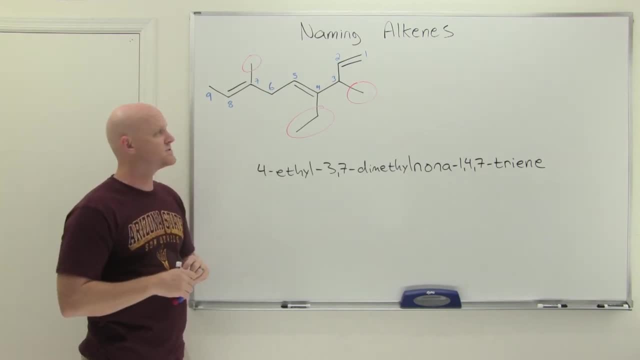 inside a small ring, like a six-membered ring, which you can't have different isomers in that case. So there's not sterically enough room for that to be possible. But then also if either carbon of the alkene is bonded into identical groups. there's no cis and trans, no EZ isomerism. 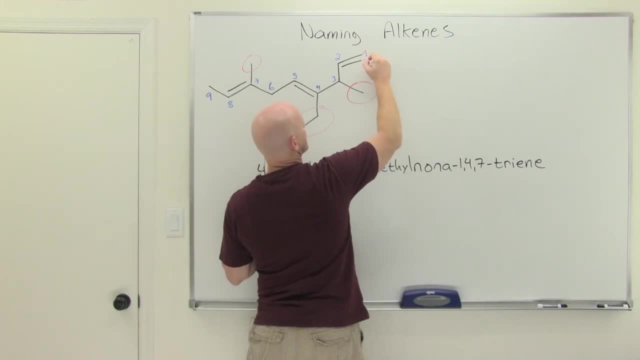 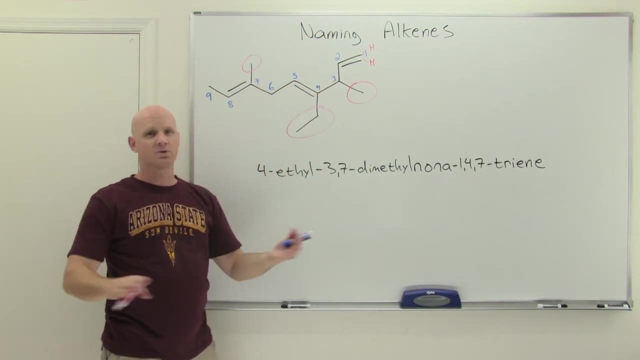 that exists, So like in this case, this carbon right here of this alkene is bonded to two identical hydrogens. There's no cis and trans, no E and Z associated with that. It only exists in one possible confirmation. So no E and Z. So, but this one right here, this carbon four. 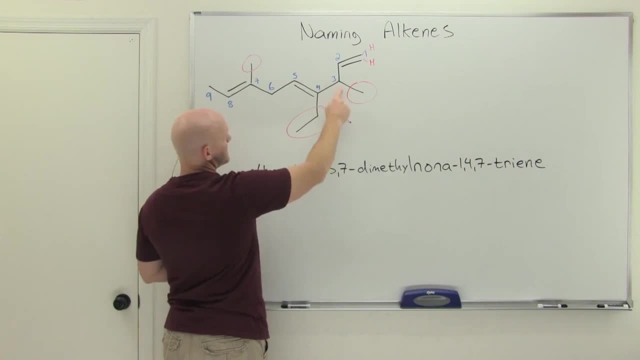 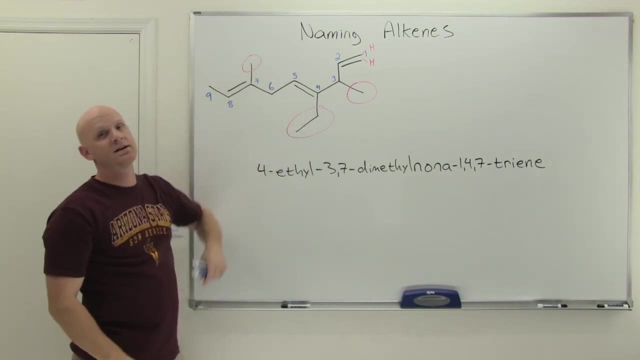 this sp2 carbon is bonded to two different carbons and they're definitely different. They're not equivalent at all. And on the other side this guy's bonded to a carbon and then a hydrogen that's not drawn in. That's two different groups, And so he's going to exhibit. 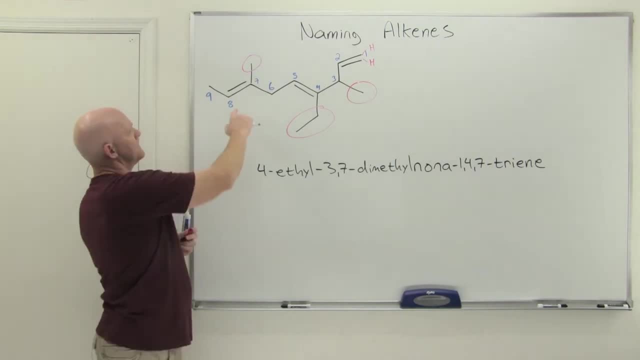 E and Z isomerism. We have to figure out which of those two we have. So go to the other. alkene here and this carbon over here. this sp2 carbon is bonded to two carbons and they're definitely not equivalent carbons, They're different. And on this side, this sp2 carbon. 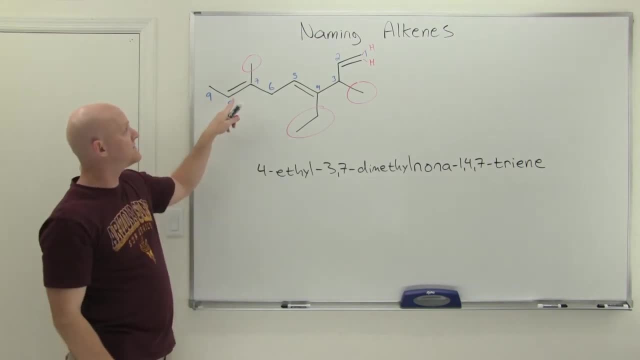 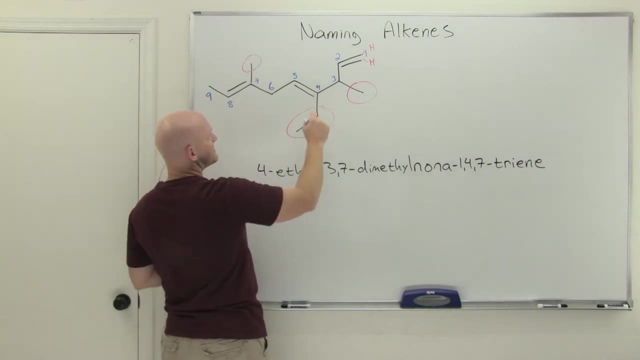 is bonded to a carbon and then a hydrogen that's not drawn in, So they're different. So he's going to have E and Z as well. So two of these two out of the three we actually got assigned E and Z- Let's go through and do that. So for carbon four: notice I circled in red. So 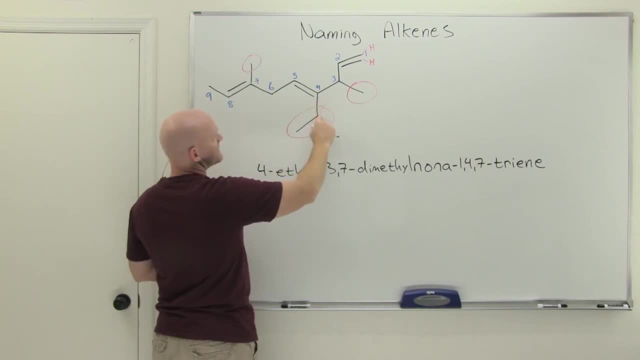 I'm going to use the blue to circle the higher priorities now, And in this case we've got this carbon and this carbon. This carbon is bonded to a carbon and two H's, So C, H, H. This carbon's bonded to two carbons and then a hydrogen that's not drawn in, So C, C, H and he's going to win. 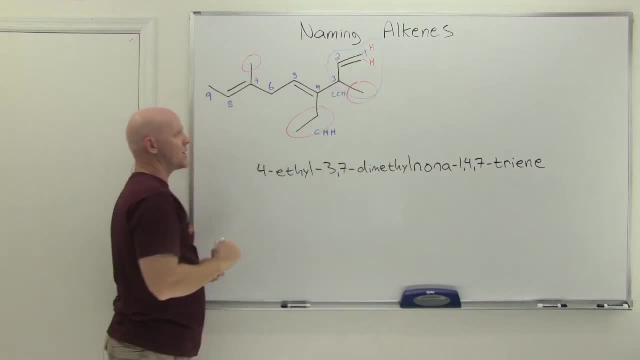 And technically I should circle the whole group he's a part of as the higher priority, And on the other side, this guy's bonded to a carbon and a hydrogen, and carbons are definitely going to win. Instead of circling the whole thing, this is going to get messy- I'll just do this. 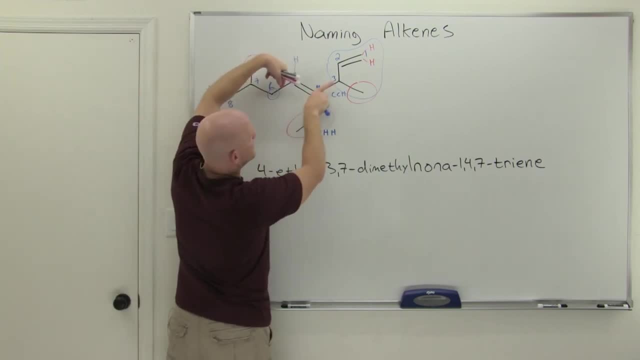 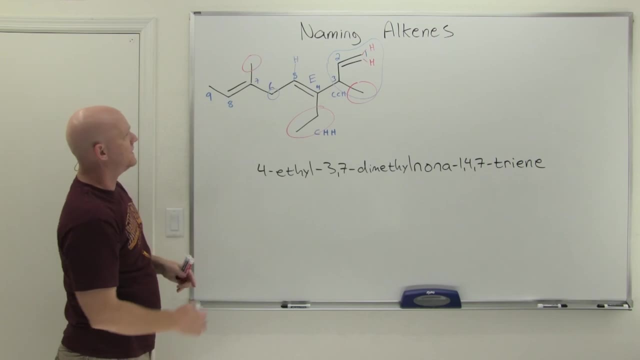 but I can see that the two groups that we've circled for higher priorities point 180 degrees apart, And that corresponds to E. And then we'll do the one at number seven here as well, And on the right we have a carbon and a hydrogen that's not drawn in, So C, C, H, and he's going to win. And 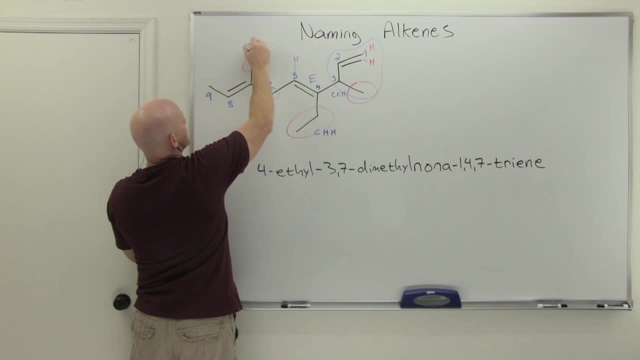 on the right hand side we've got two carbons: This one's bonded to three H's, This one's bonded to a carbon and two H's and going to get the higher priority here as well. So I'm circling it again for this guy, And then on the other side, this guy's bonded to a carbon, and then